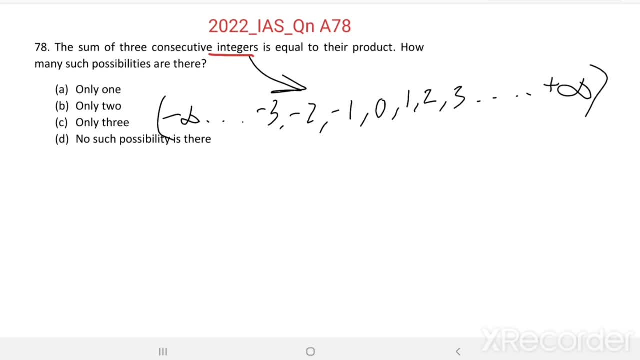 All these are integers. Here we have to find how many possibilities are there? Well, sum of three consecutive integers is equal to their product. Let us take three integers as three consecutive integers, as x minus 1, x and x plus 1.. This 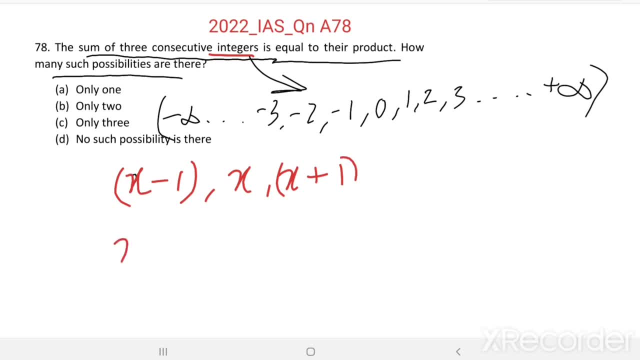 is three consecutive integers, Then their sum equal to x minus 1 plus x plus x plus 1, which is equal to their product. x minus 1 into x, x plus 1.. Then x minus 1 plus x plus x plus 1, equal to 3x, which is equal to x minus 1. 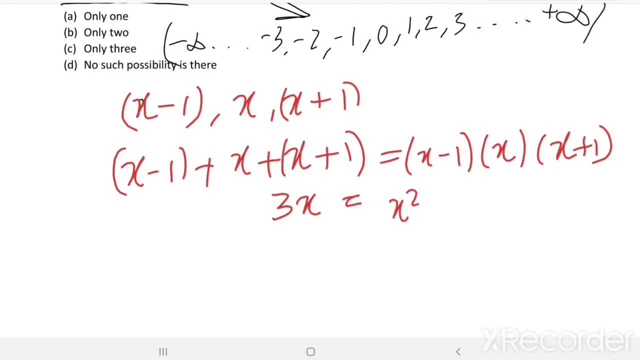 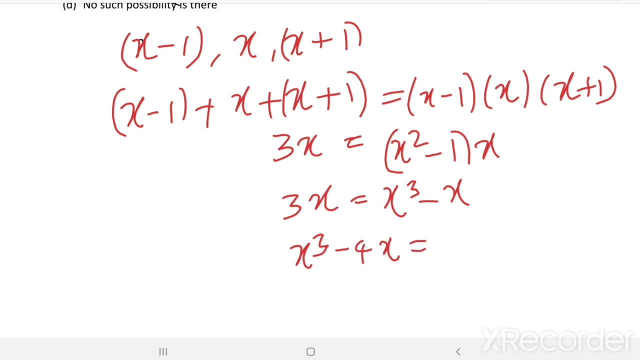 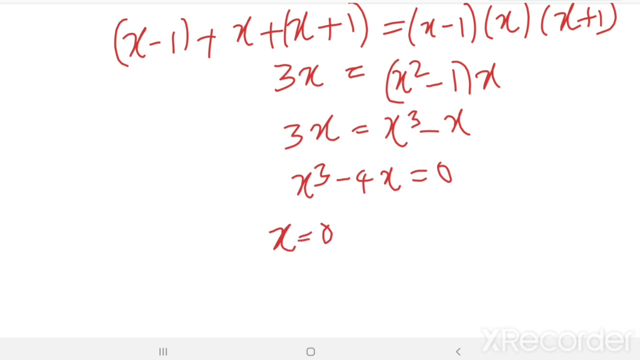 into x plus 1, equal to x, square minus 1 into x. Then 3x equal to x cube minus x, x cube minus 4x equal to 0.. From here we get x equal to 0 and x square equal to 4.. From this we get x equal to 2. 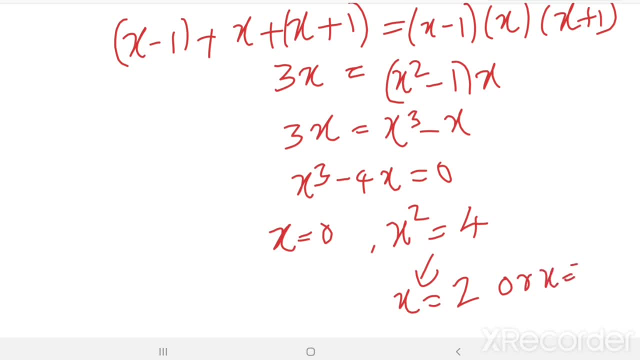 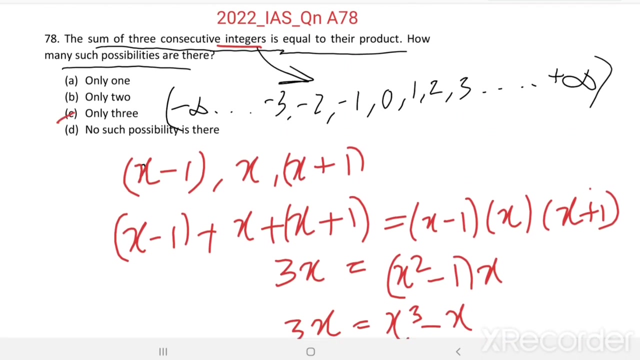 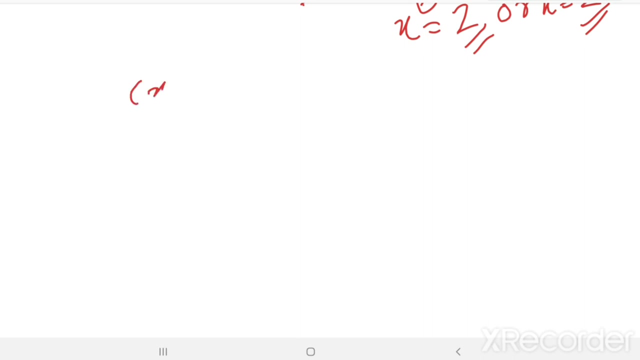 or x equal to minus 2.. So x can take three values: 0,, 2 and minus 2.. That means there are three such possibilities. Option c is the right answer. Now. c: We took x minus 1, x and x plus 1, x plus 1 as three consecutive integers. When: 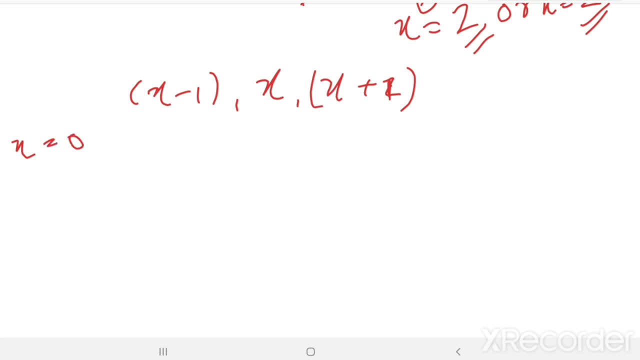 x equal to 0, x minus 1 equal to 0, minus 1 equal to minus 1,, 0, then 1.. There are three possibilities. They are sum equal to 0 and their product equal to 0.. When x equal to. 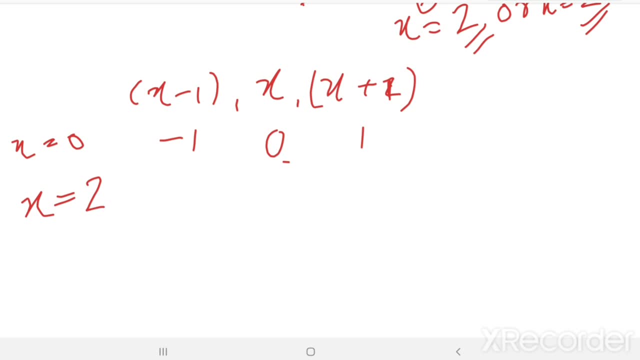 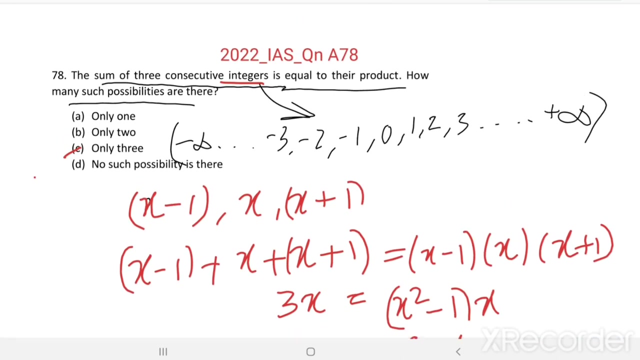 2,, here 1, then 2, then 3.. When x equal to minus 2,, here it is minus 3.. Here it is minus 2.. Minus 2 plus 1 equal to minus 1.. So there are three such possibilities. The solution: